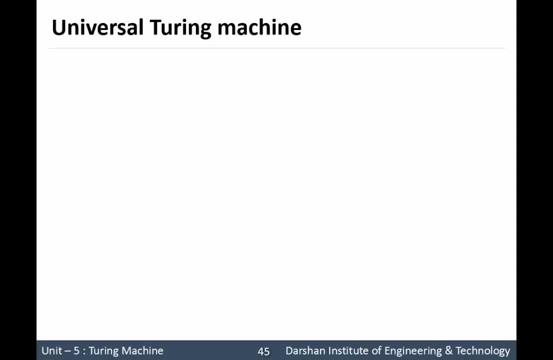 So to understand that, let us take an example. So we have the language, a subscript of tn, N, w, where n is Turing machine and n accepts the string w In Turing it coordinates the string. So this language atm has 2 elements. 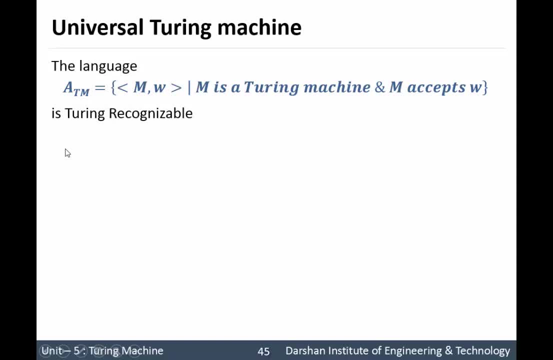 1st one is m, that is the Turing machine, and w is the string. If we pass into the Turing machine, m will be accepted. So if we have string w which we will see that we have heard this string a passed, so this Turing machine M is accepted, then we can say this whole thing is 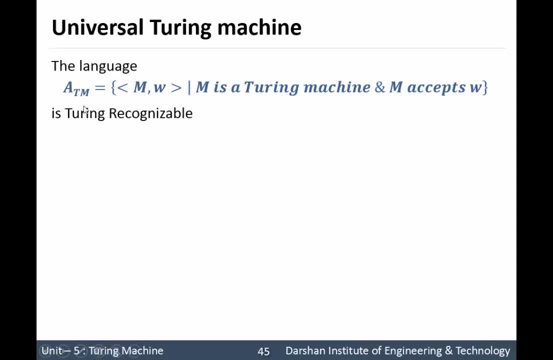 lanced into the language KTM and we can say this language is Turing recognisable now. if we change this string W, then Turing machine M may accept this string, sometime may reject this string or sometime it goes into the loop. so we can say it is Turing recognisable but not be decidable now. given description of a. 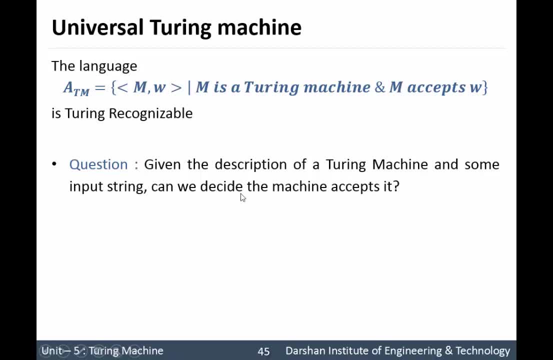 Turing machine and some input string, can we decide the machine accept it. so here is the role of universal Turing machine from into plane. so in universal Turing machine we can pass the description of other Turing machines and some inputs. so pass description of another Turing machine along with some value of. 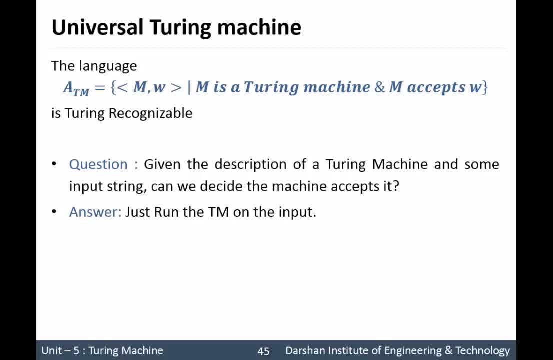 Turing string to universal Turing machine and then run it. Now universal Turing machine will behave exactly like other Turing machine that we have. So here is the possible results. So if the Turing machine M that we have accepts the W, then our universal Turing machine will. 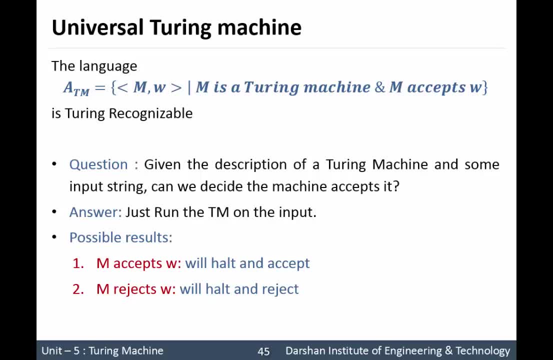 halt and accept. If M rejects W, then our algorithm, that means our universal Turing machine, will halt and reject. If M loop on W, then our algorithm will not halt. So universal Turing machine will exactly behave same as Turing machine M that we have passed to it In source. we will. 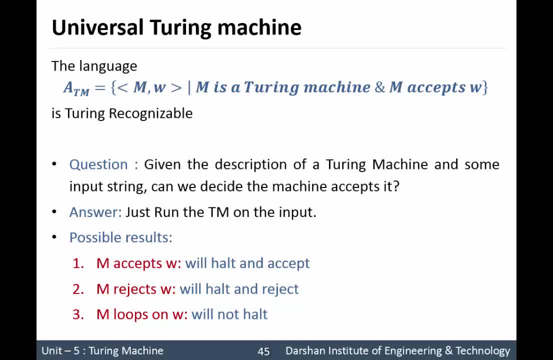 pass Turing machine M in input string W to universal Turing machine and we will see how universal Turing machine behave. So we know that how the universal Turing machine behave, it behaves exactly same as how the M is supposed to behave. So here are some of the option. 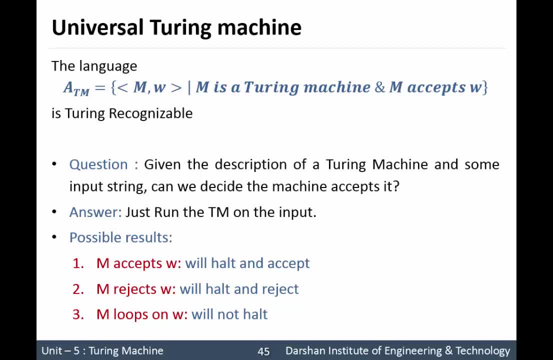 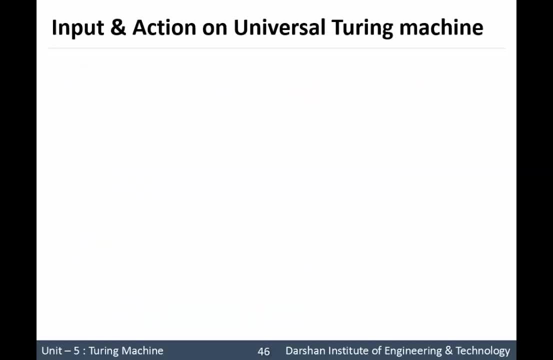 it could either halt and accept, or halt and reject, or sometime it may not halt. Now let us see what is the input and action we can have in Turing machine. So input of universal Turing machine is the description of another Turing machine, M, and input string of universal. 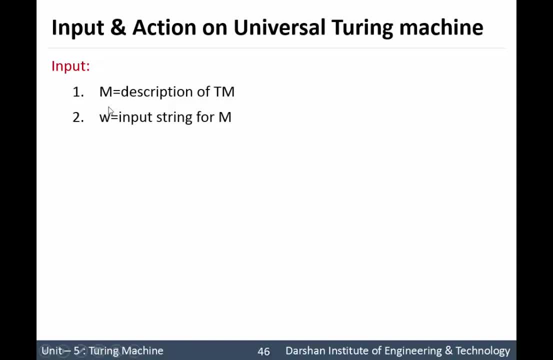 Turing machine M. So this two will be passed to the universal Turing machine and the action that can be carried out by the Turing machine is first. one is simulate the M and second one is it behaves just like M. So sometime it may accept, sometime it may reject, or sometime 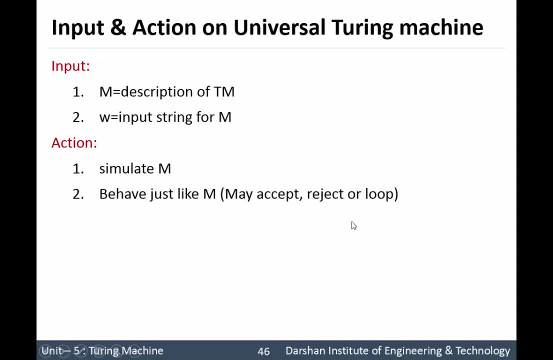 it may not. To understand universal Turing machine in better way, let us compare our universal Turing machine with general purpose. We know very well what is the general purpose computer do. In our general purpose computer we write our program and then our computer will help us to run that program. For example, 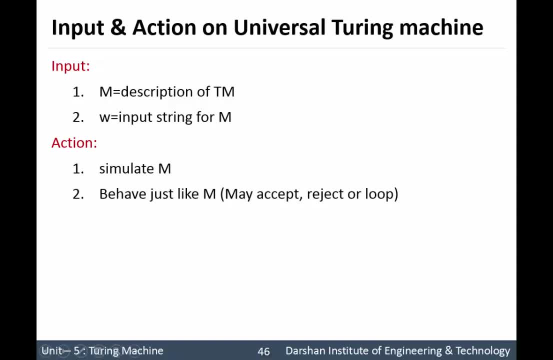 we have written a program of to check whether given number is prime or not in some of the programming language. So consider: your program is first Turing machine M, you put your program in your computer. then put your program in your computer and then put your program in. 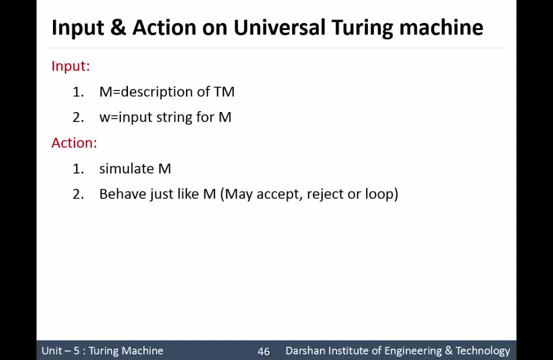 computer run your program and it will give us the output base on the input you have given. So here your program is some Turing machine M and your computer is universal Turing machine. I hope now concept of universal Turing machine is clear. So in last we can say universal. 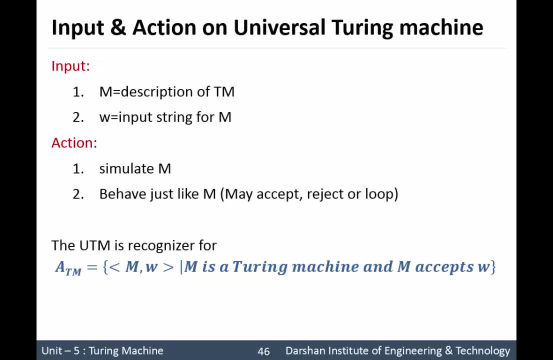 Turing machine is recognizer for the language, a subscript of T, M, M, W, where M is Turing machine and W is string of M. So for this language universal Turing machine is recognizer. It is recognizer because sometimes it may accept, it may sometimes reject and 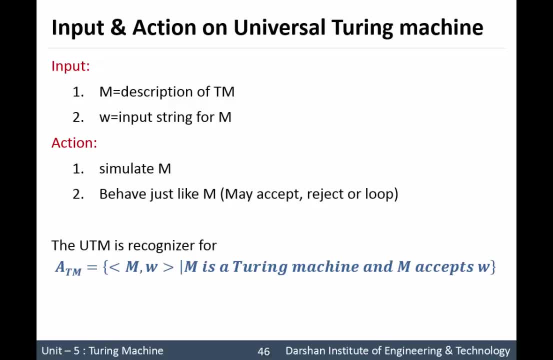 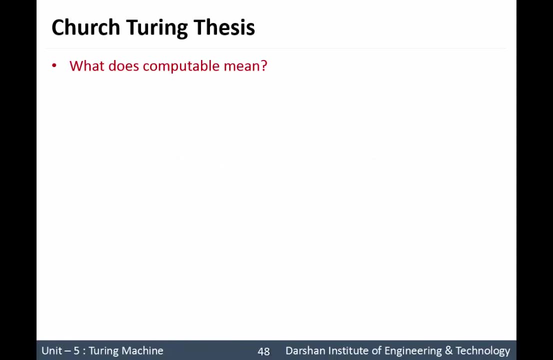 it may sometimes look differently upon the Turing machine and the input. So this is the concept of universal Turing machine and how it works. I hope it is clear. Now let us discuss church- Church during thesis. Church during thesis is comes from the question: what does the computable 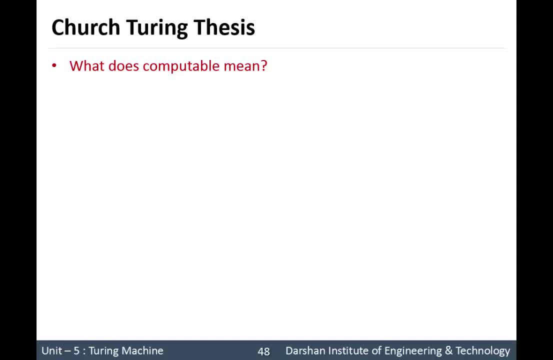 mean. In old days, term computable was actually fuzzy. We cannot give proper definition. in order to define, what does computable mean? Meaning of term computable was given by one American mathematician, Alain George Church. He came up with the idea of lembran calculus. 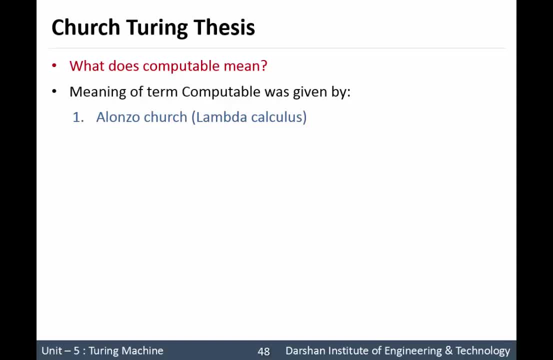 So lembran. Lembran calculus was a kind of machine that could perform some computation. So whatever can be calculated by lembran calculus, that is called computable. And later on another computer scientist, Alain Turing, come up with the concept of Turing machine. So Turing. 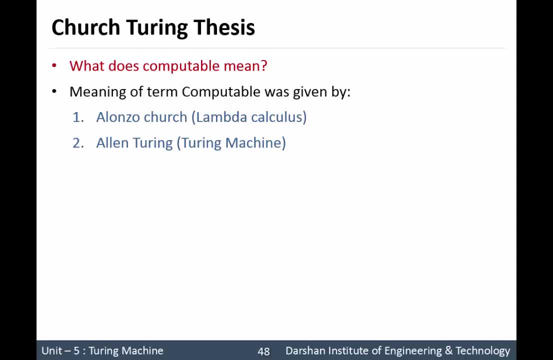 machine is again another kind of computation model that is used to perform some computation. So what was this people come up with this idea? So what was this people come up with the idea of lembran, calculus and Turing machine And then state that whatever they computable 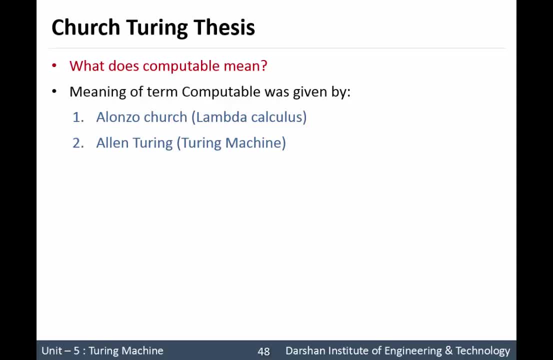 by this machine- that is what we can call, is computable Turing machine- and lembran calculus is equivalent in power. So they work in different weight but they are equivalent in power. But actually we do not use lembran calculus as the benchmark to standardize the computable.